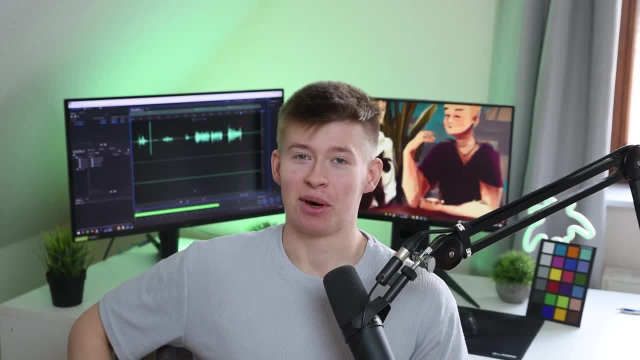 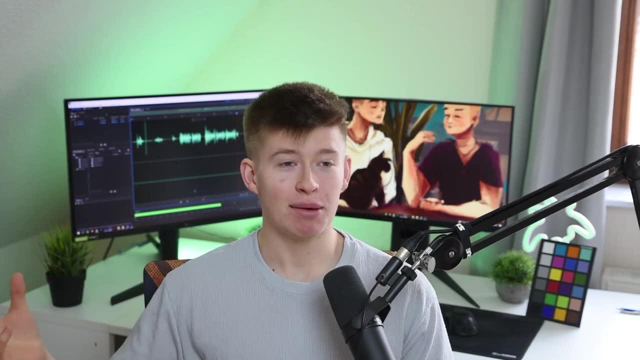 Hello and welcome to what the video title says. this is: We're going to implement a Redis cache together with a database so that we nicely distribute the workload between the database and a super fast caching layer with the example of Nextjs. but this really works in any framework in. 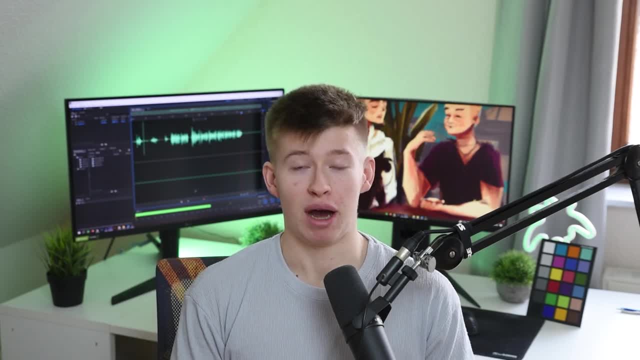 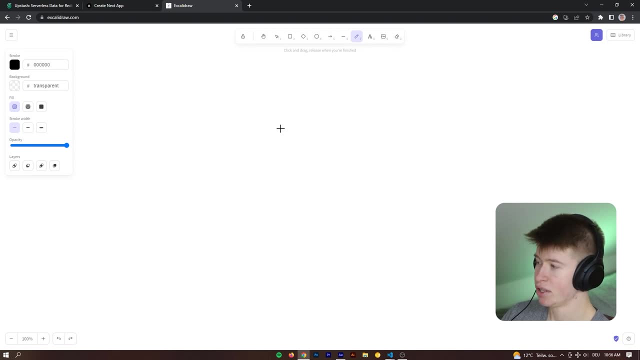 JavaScript or even in other languages such as Python. So really quick, before we take a look at how to implement a caching layer with Redis, let's very briefly talk about what Redis even is. You've probably heard that Redis is an in memory database, meaning in memory, you know. 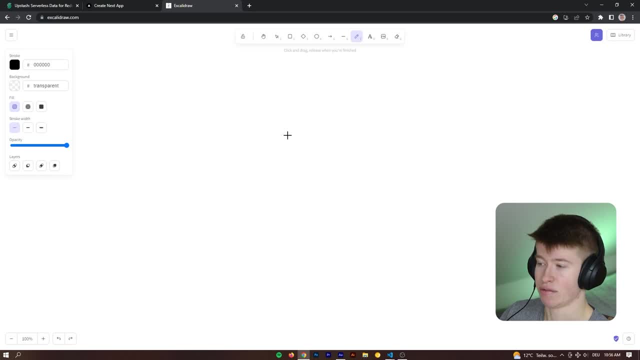 when you declare a constant in JavaScript, that's basically saved in memory, So it's not persisted anywhere. But Redis also persists to the disk, So you could even use it as an actual database. So say, you have the client right here, the user client. the client makes a request currently. 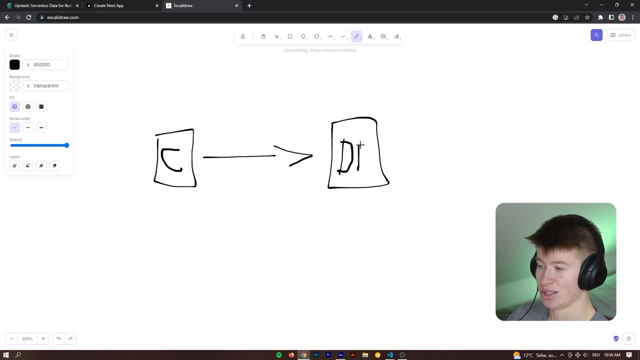 to a database, the database lives over here And then the database returns the data back to the database client. that's the architecture when we are not using Redis and want to persist data And notice how the client makes a request to the database every time. 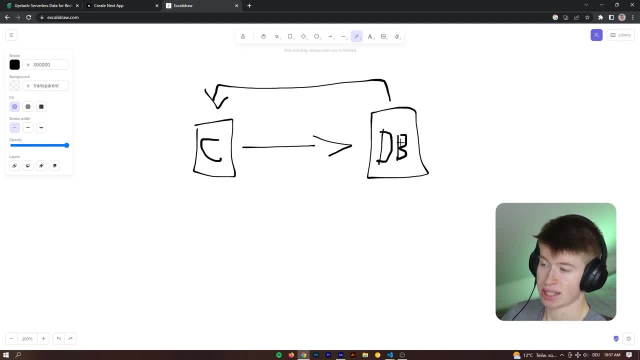 So the workload is not distributed at all And the database has to serve every request with the according queries to the database And depending on how large the database is, that can cost you a lot of quota on the database. With Redis let's go down here. 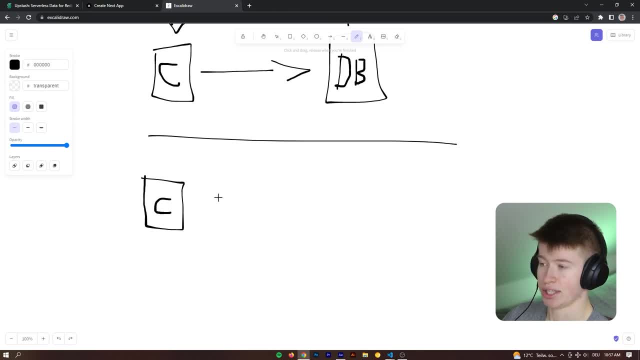 the architecture is a bit different. So we have the client right here And then the client makes a request to the API route. Obviously, the API route is called up here too, but it always calls the database, So it doesn't really make sense putting it in there. But the client makes a. 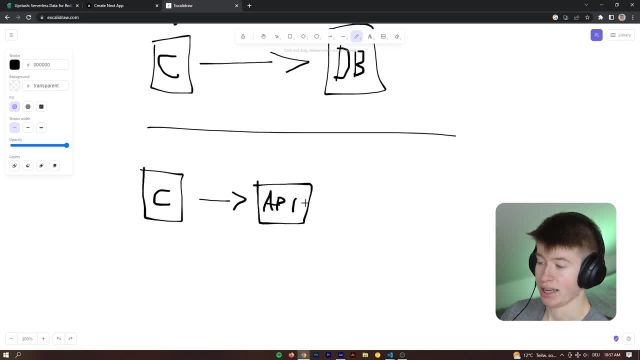 request to the API endpoint that we define. And the API endpoint now checks: is the data already in Redis, So in our caching layer, or is it not? let's move them a bit like that: So the API checks with Redis, Let's say, Redis lives up here, this is Redis. The API checks with Redis- do you already? 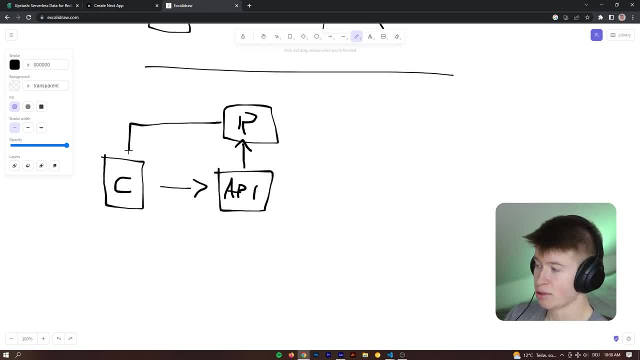 have this data in your store, And if you do, just send that back to the client right away. And if you don't have it in your store, then so this is going to be a wife or yes, And if you don't already have the data, so that's going to be no. Only then are we going to query the database. 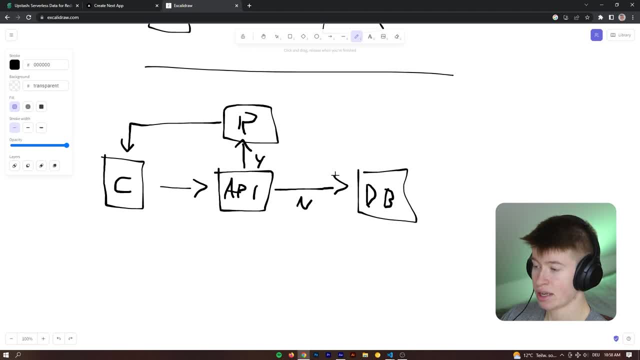 And whenever that result from the database comes back to the API route, like that that is being put into Redis. So for the next request we make to the API route for the same data, the database is not going to get queried, But instead this query right here, the Redis one is going to return. 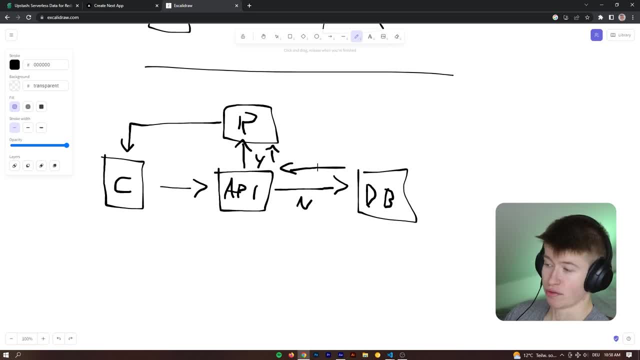 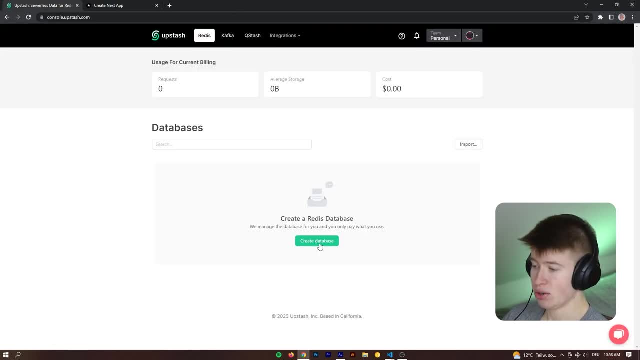 true, it's already going to be in Redis, so that the request will will be soft, faster and without putting any workload on the database whatsoever. That's how Redis works, And let's now implement Redis in practice. we're going to be using upstash for this. Now, upstash is just a service that. 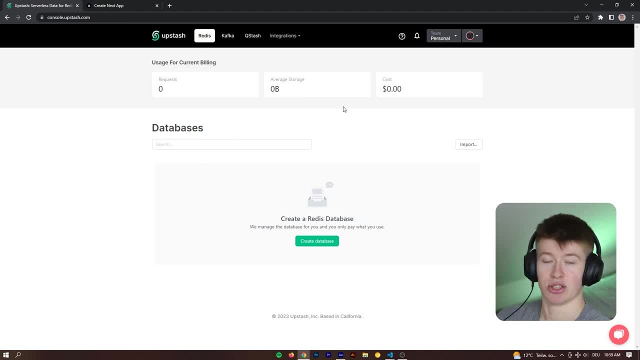 manages Redis for us and gives us a very nice CLI to interact with and handles also scaling of Redis for us. You don't have to use upstash I'm going to do in this video, because they make it very convenient to work with a Redis database. 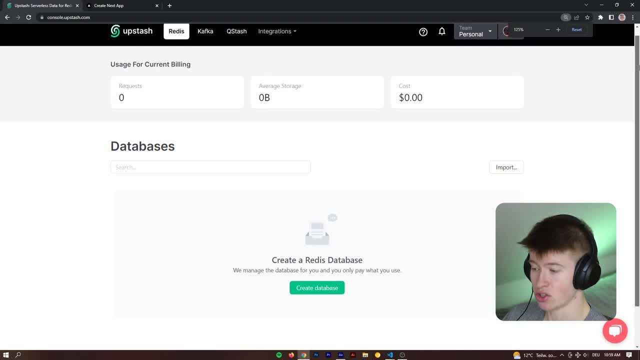 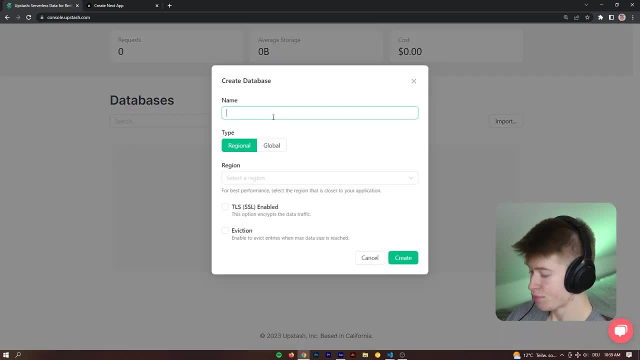 If you want to follow along using upstash, be sure to make an account. This is not sponsored, by the way, I just genuinely like their service. And then let's click the Create database button. Let's call this caching. This is going to be a regional database And I'm going to host this. 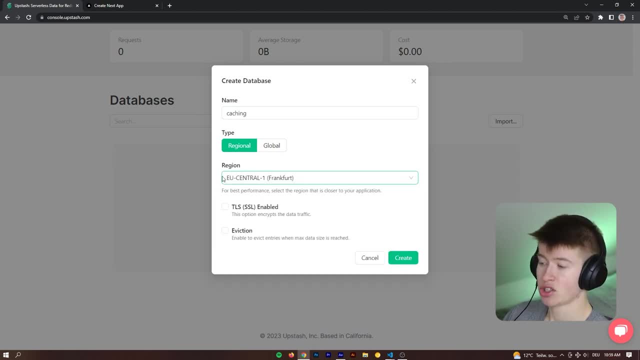 close to me, which is an EU central one. you would want this to be as closest to your users as possible, not necessarily closest to you. we are going to enable encrypt traffic, And then let's click Create or Redis database. Now the UI is very clean. 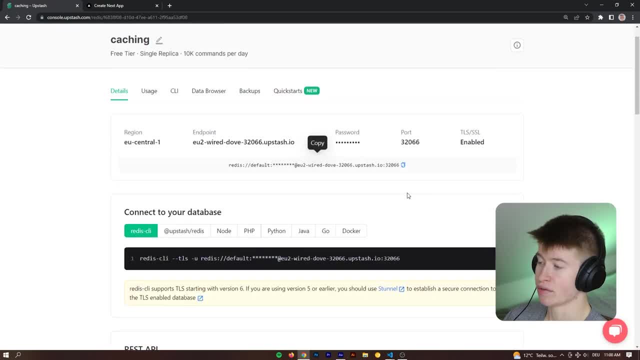 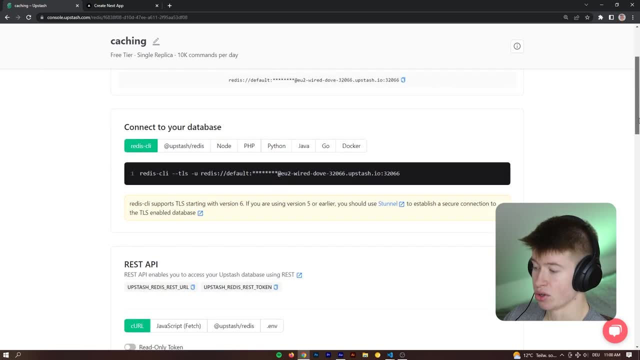 the database is being prepared for us And that's literally all we have to do Now. we got our connection string And that is the string we need to connect to our Redis database could also use different methods, like the two different environment variables declared down here, But we 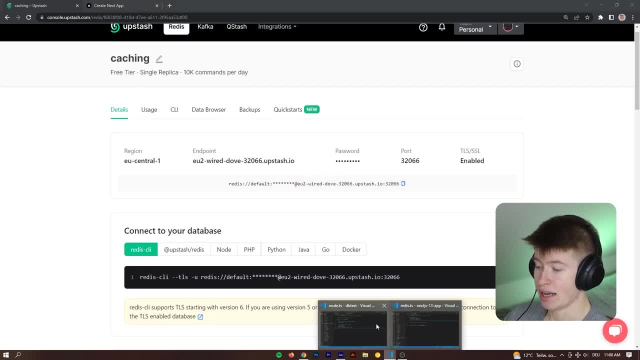 are just going to copy the connection string right here And then let's go into our app. Let me zoom in So you can see the string, And then let's go into our app. Let me zoom in so you can see the string, And then let's go into our app. Let me zoom in so you can see the string. And before: 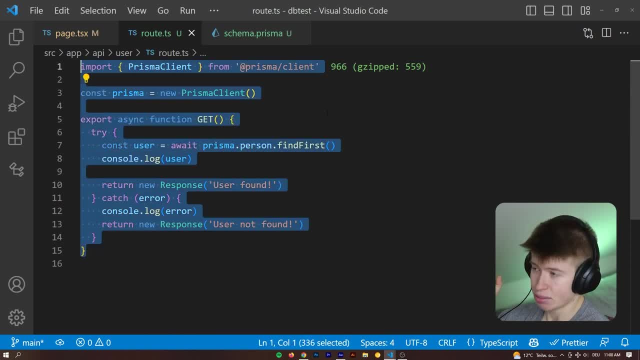 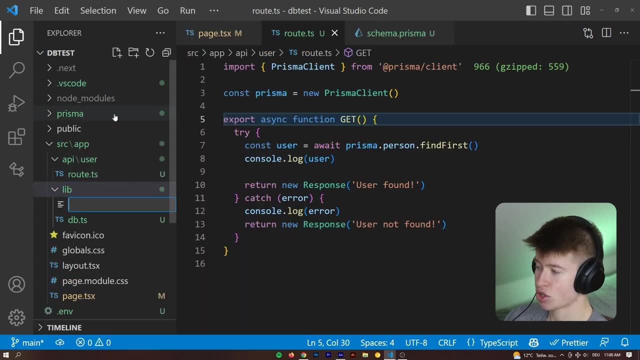 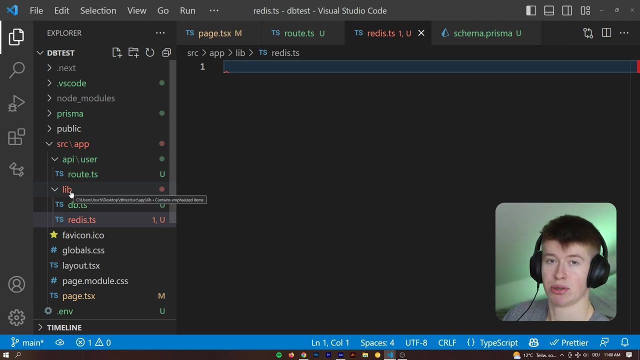 getting into the database code of what I've just showed you as a concept. let's first initialize a Redis instance right, And to do this we can go into our lib. Let's create a new file and then call this: Redis dot ts. Now, the reason I'm doing this in a folder called lib is because lib is. 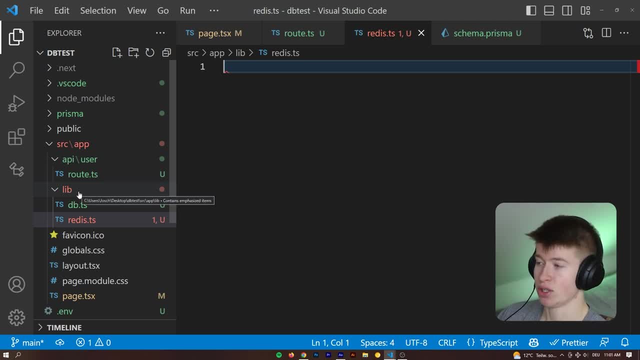 usually used for preparing libraries to be used in your project. And now let's get started with creating or Redis instance, so that we can then use it in our application to make everything more performant. And the way we do this is by first installing a dependency. 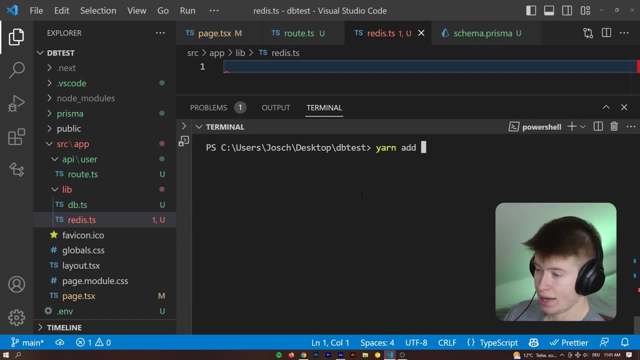 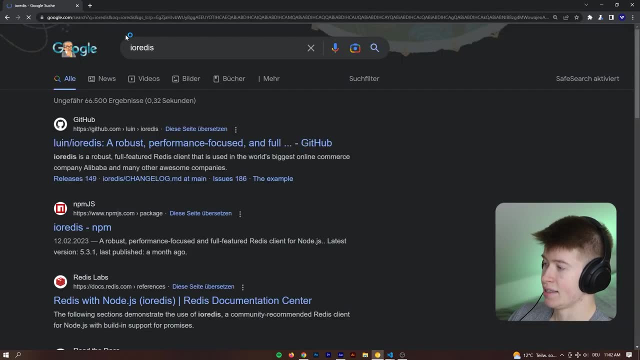 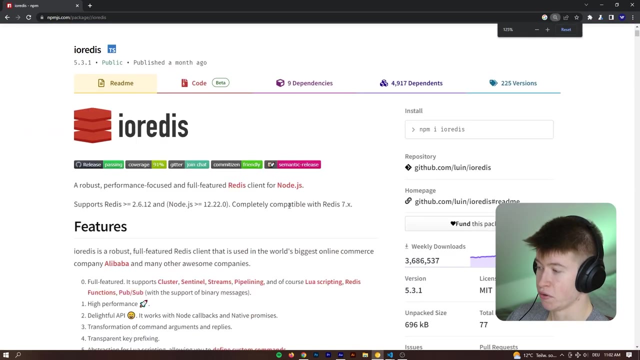 That dependency is called yarn add or npm install. I owe Redis. I owe Redis- if you don't know yet, is a package. I own Redis. Let's go ahead and check it out. on npm, really quick, It's a Redis client for node js So it can be used on the server side. got a bunch of installs. 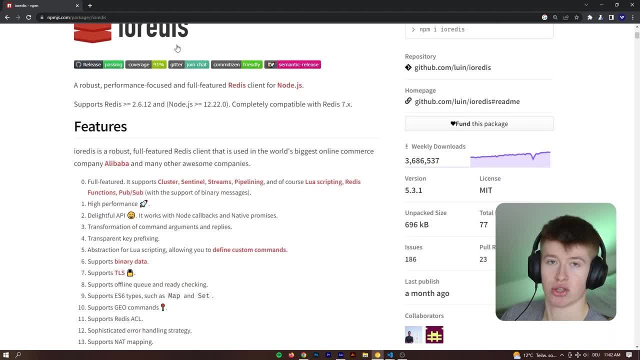 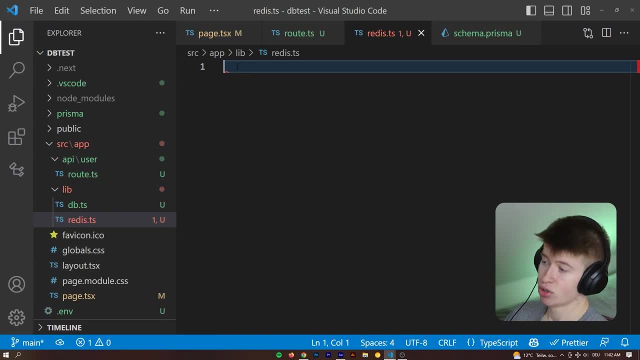 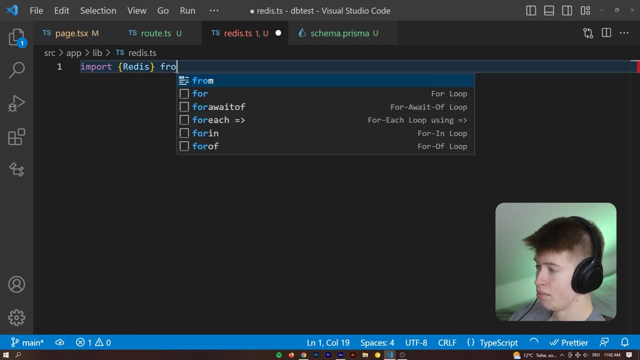 So many people are using it. It's high performance. it's pretty nice to use. We are using IO Redis for this. we can start the dev server backup And now, because we've installed that dependency, let's close that down. we can say import and then read this from IO Redis And 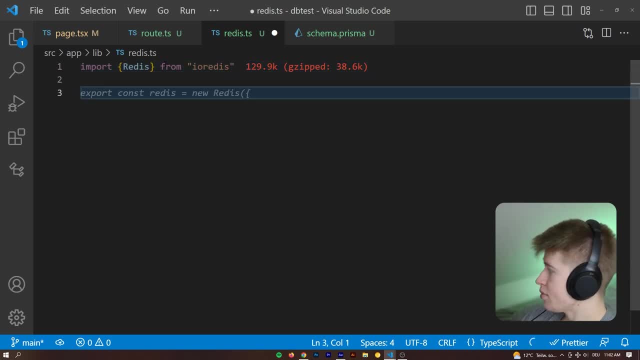 that is what we're going to use for Redis client to initialize it. Now. to initialize the client, we can write a little helper function called get Redis URL, And the only thing this function is going to do- and let's disable GitHub Copilot for this- is give us back the 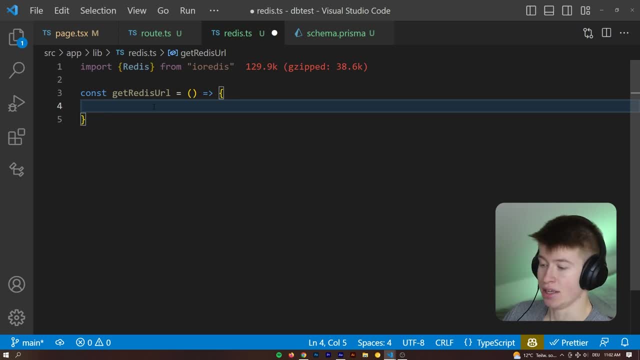 environment variable that we have set for the Redis connection string- the connection string- remember that we got from upstairs. we want to save this as an environment variable because it is a sensitive piece of information And we don't want to leak to the client side. That's why we are. 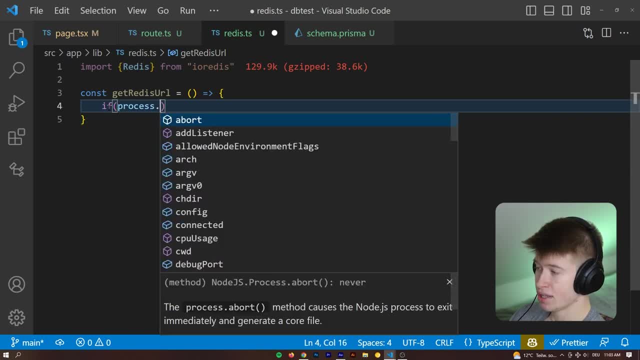 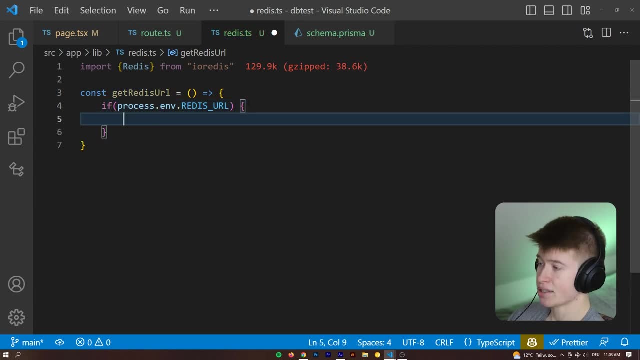 putting it into an environment variable. If the process dot env, dot Redis underscore URL, this is what we are going to call this connection string. If that exists, then we are going to return that process dot env, dot Redis URL. And this is only going to be true if we are on the server side, right? If we're on the client. 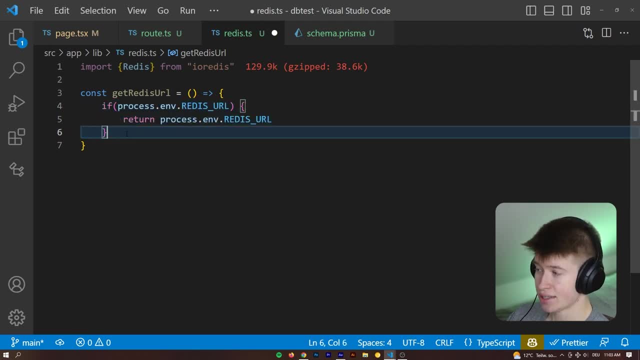 side, this process, dot, env. dot. Redis URL is not going to exist, And that is in our best interest. So if it doesn't exist, we're going to throw a new error And this can say whatever you want. Let's just say Redis- underscore URL is not defined, And then to initialize our clients. 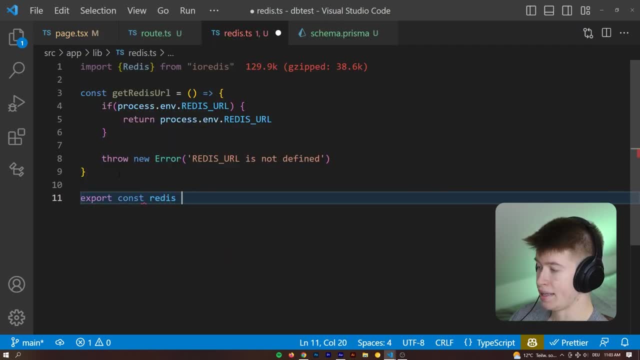 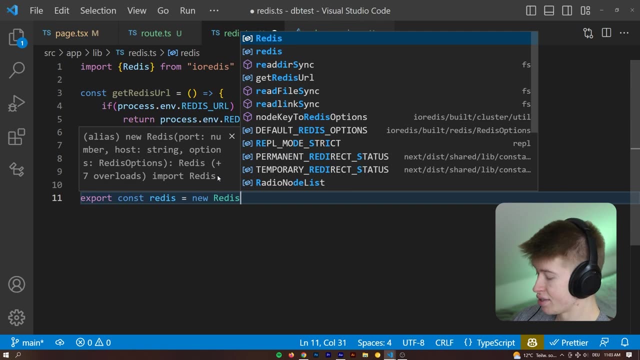 all we need to do is say const Redis and export that. So export const Redis is going to be equal to. and then a new Redis. What do you want to do? I'm going to say const Redis And then you read this: we've imported up here from IO Redis. and then pass in the get Redis URL and invoke that. 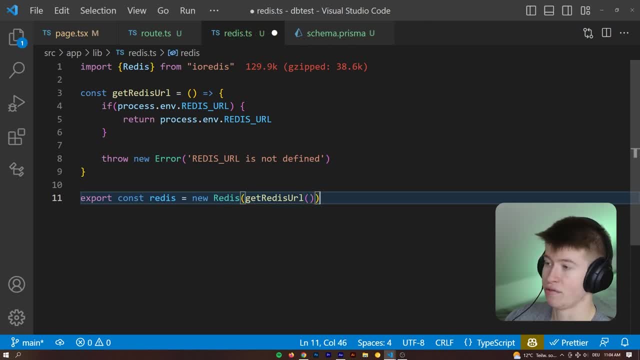 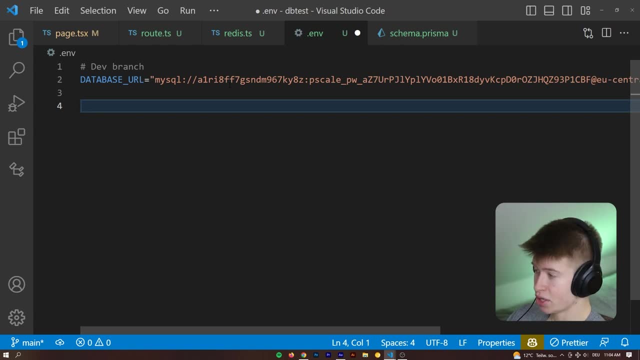 So that is going to give us back or process dot env. dot Redis URL, if it exists, And if it doesn't exist then it's going to throw an arrow so we know what's going on. And now in our dot env we're going to declare the Redis underscore URL as the string we have just copied from upstash. 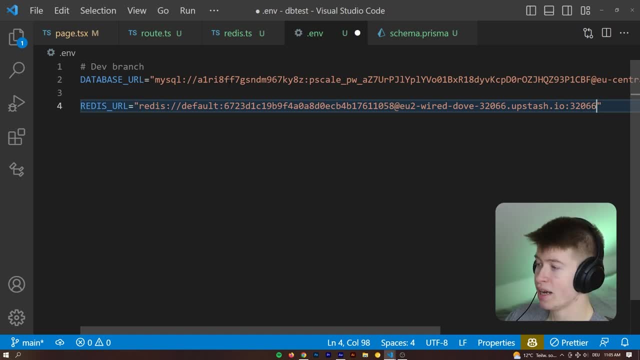 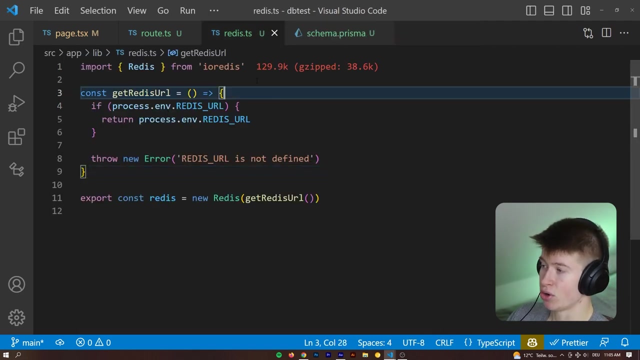 Now, because we have enabled encrypted traffic earlier. remember we want to put a Redis with a double s right here. So, just like HTTPS or WSS for secure web sockets, This is the way that handles secure Redis connections, And now we have enabled our client and are ready to work with it. 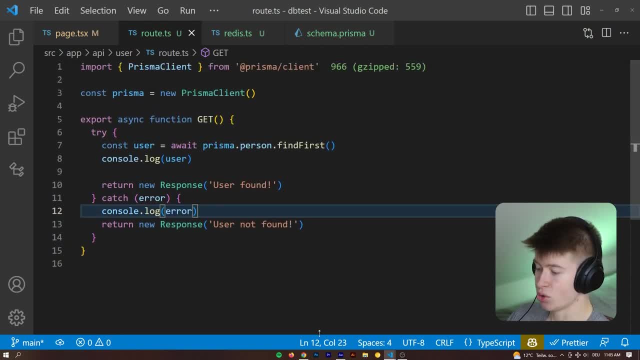 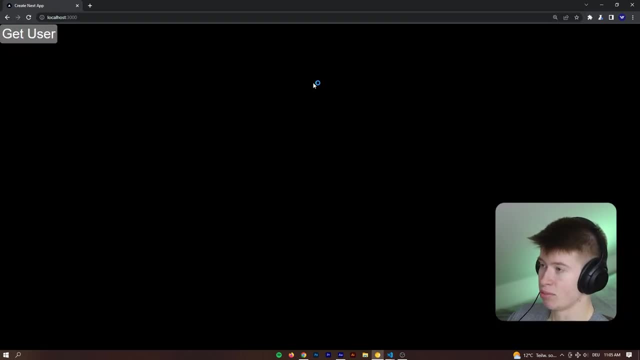 Before we get to use the client, though, Let's first take a quick look at this app right here. Let me pull up the server, And then there's one single button. Let's have the side by side, that's a bit easier for you to see. There's one single button in this app. 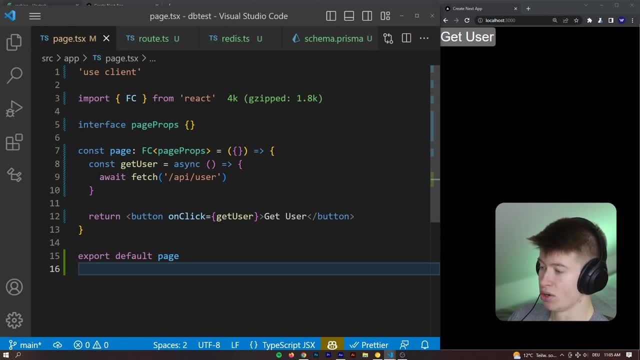 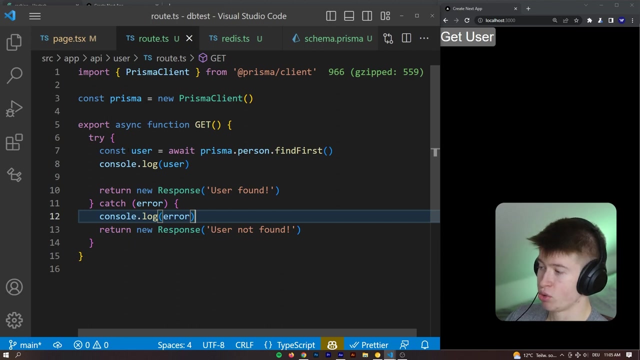 And that is the get user. When we click this button, an API call is made to the slash API slash user. It doesn't matter whether that's a node js, API, Ruby Python, this truly doesn't matter. I go, I went with node js And then, inside of this folder, we are just querying our database to find. 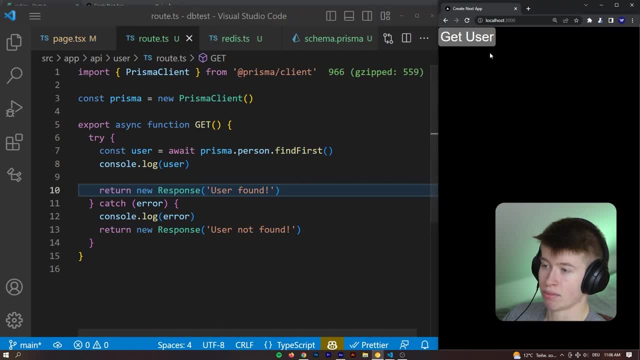 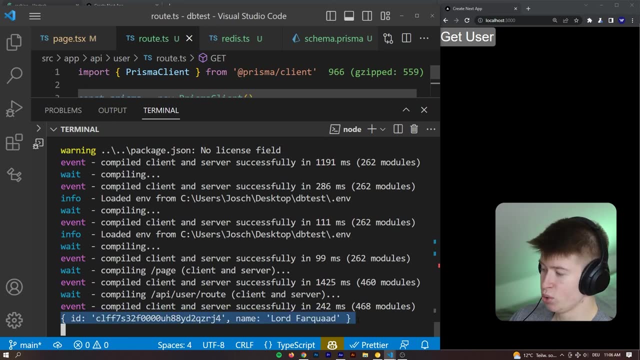 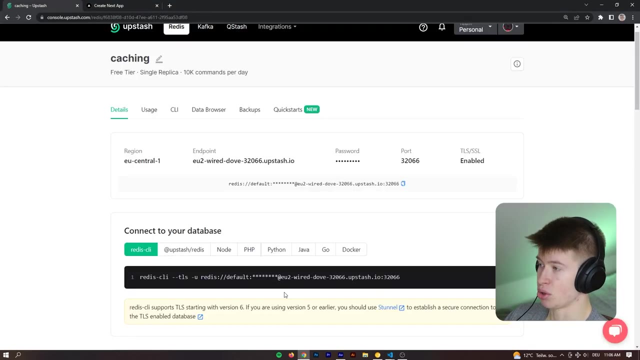 a user logging that out and then returning some kind of mock response. So when we click this button and take a look at the console, we can see in the console we have found this user with a new ID and the name name of Lord Farquaad. from our database And in the concept view that I showed, 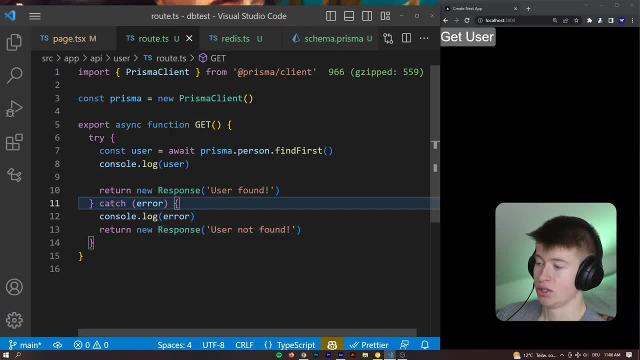 you earlier. well, I don't have it open anymore, But you know this would be. the database is always queried without any caching involved And that's not optimal because you're not distributing the workload even if you already know the response. right, because you've previously gave back that. 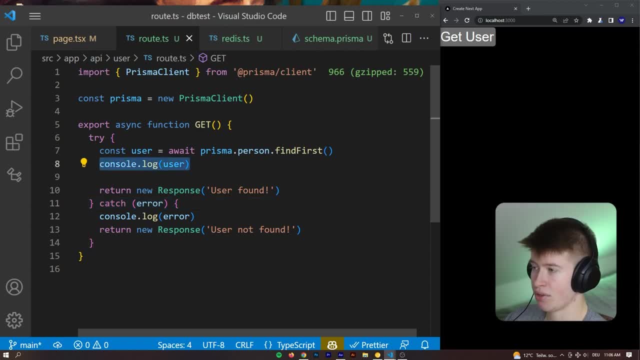 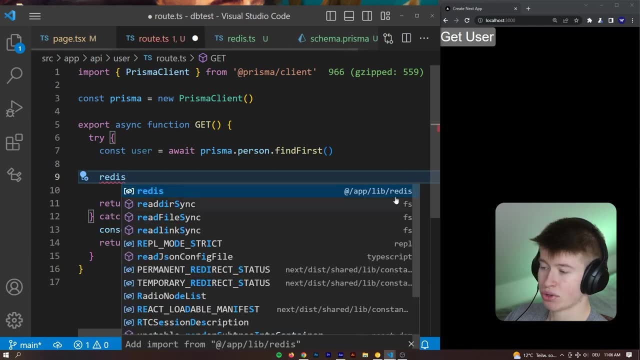 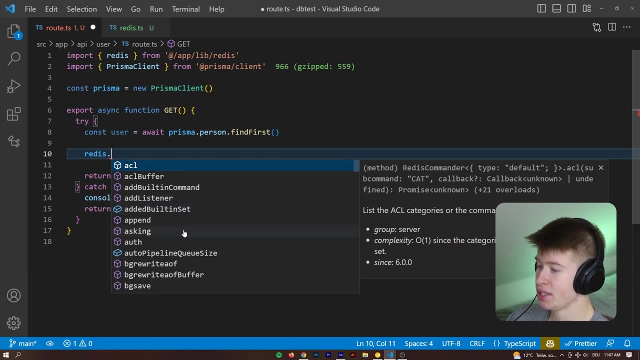 response. So it just makes sense to cache that. And now the way we cache that with Redis is super easy. We can say Redis read this and import that from our, from the lib file we have just created. And if we take a look at what we can access on this Redis property, there's a bunch of stuff we 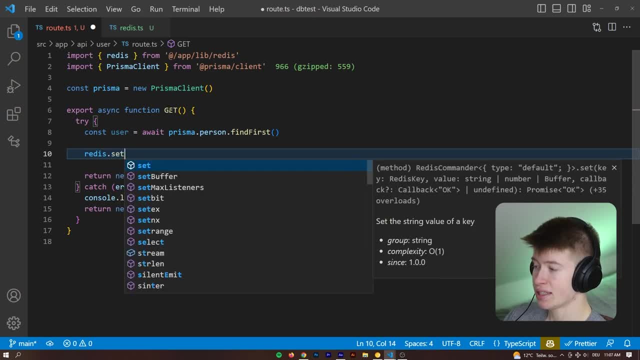 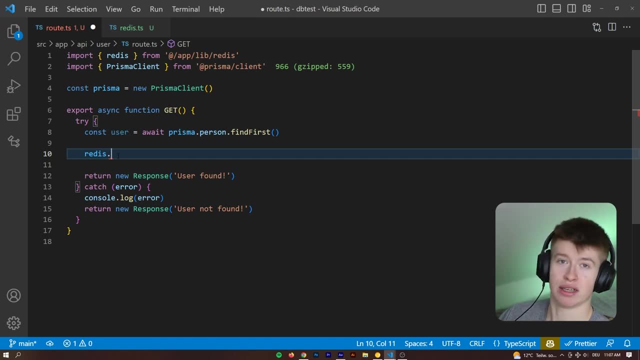 could use, right, But the most important things are the set and the gets, And they do exactly what they promise. With Redis dot set we can put new values, key value pairs, into our database, So that means we could say Redis dot set. Hello. 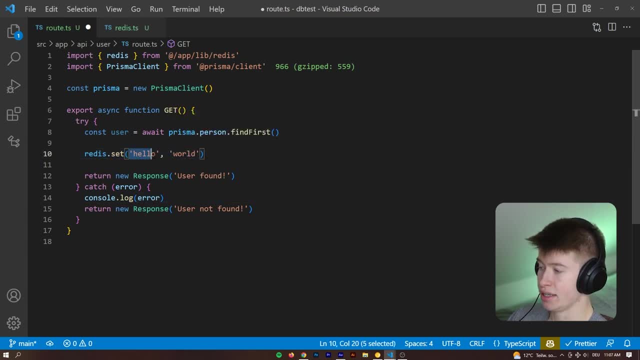 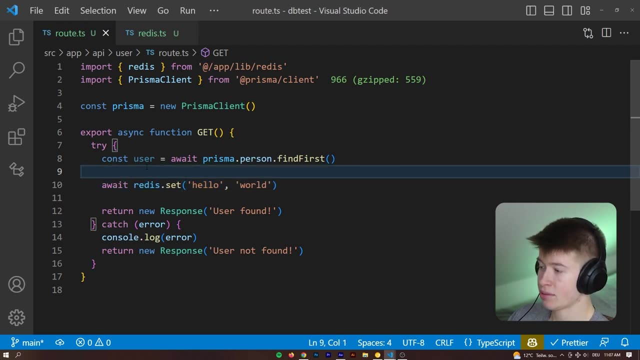 and we want Hello to be of world right. So this is the key, And world would be the value that we save, along with a key. Normally we also want to await that, because that is an asynchronous operation. And now let's try pressing on the button once again and seeing if it worked. 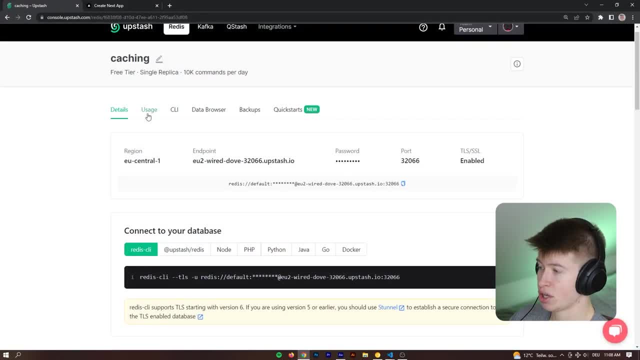 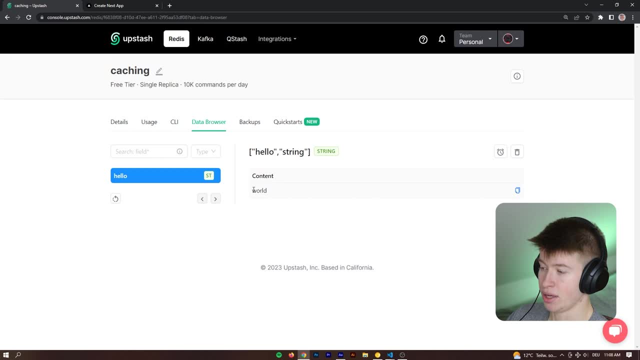 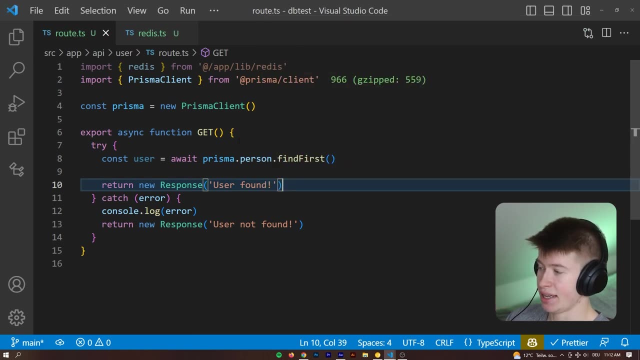 we didn't get any error. So let's go into our upstairs data browser And now we can see we've successfully created a string Hello, with the world content inside of it. Okay, so now that we know how to use Redis, let's see how we can optimize this back end. 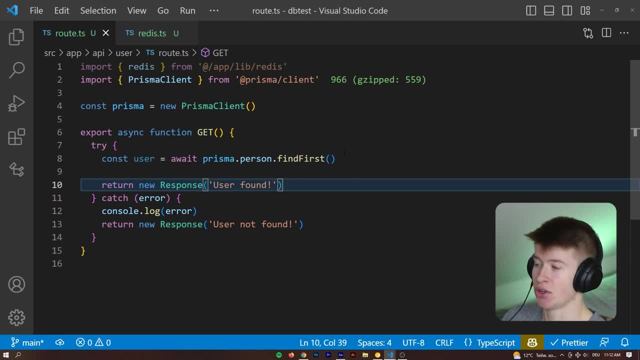 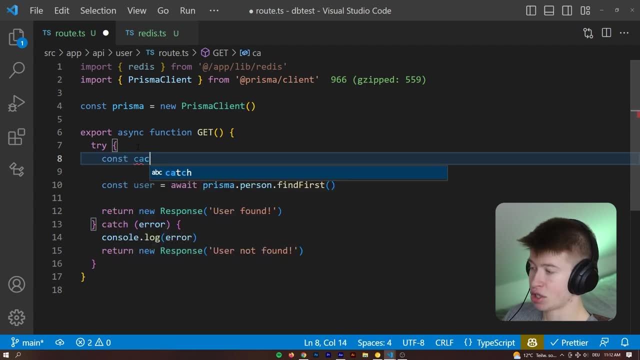 And we only want to query the database if the value is not in the cache already. right, So to check if the values in the cache already, we could say cons cached value is going to be equal to Redis dot get, because that's how we get values from the database. And then we want 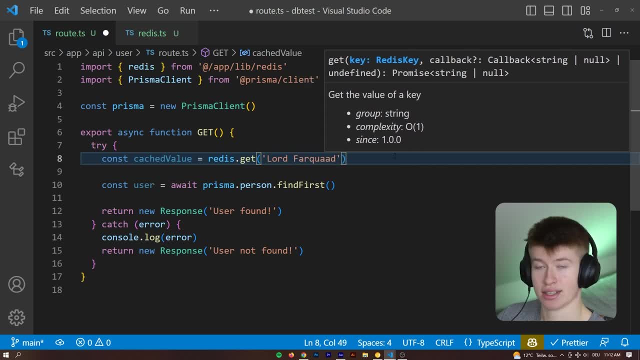 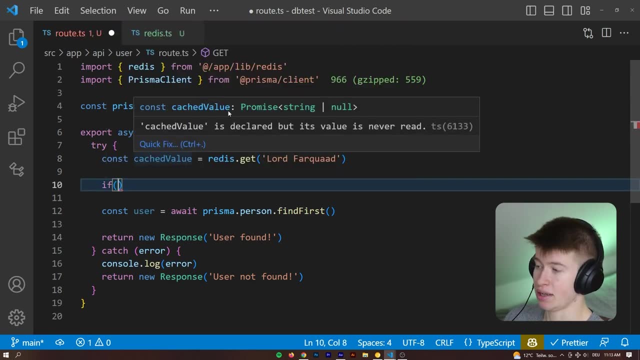 to check if the user Lord far quad already exists in or Redis cache And if that user already exists, if this query was successful, because it comes back as either a string or no, And obviously we also need to await this operation because it is asynchronous, So we get. 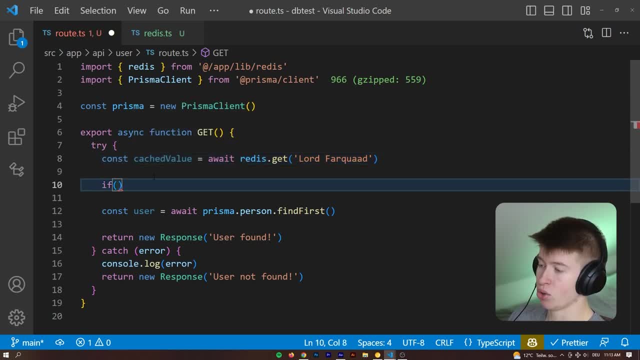 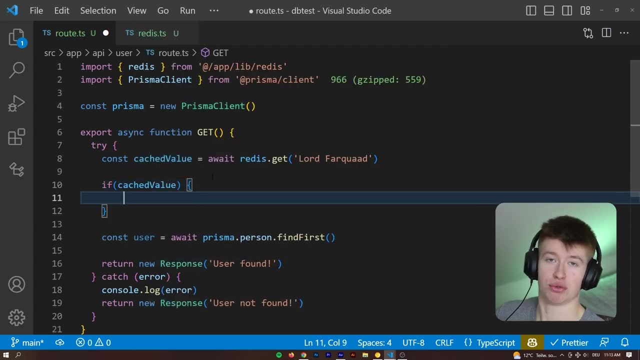 back a string or null the string in the success case and no if the Lord far quote value is not found. So if we have have a cache value, then that means we can just return that to zero to the user. there's no need to even query or database So we can say return new response. 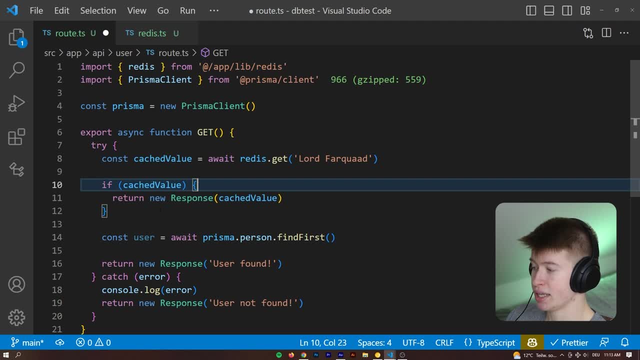 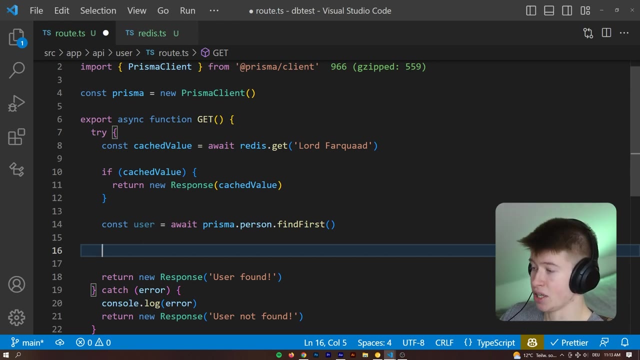 And then here we can give back the cached value of lord farquad. and if that doesn't exist, if the cache is not populated with that value, only then are we going to actually query the database. however, if we query the database, we want to ensure that this result is also stored in the cache, right, so we can say: await redisset. 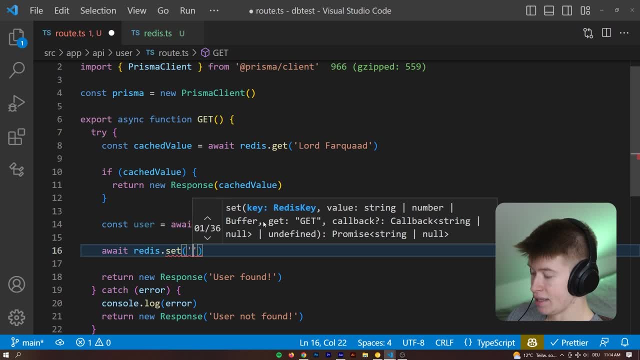 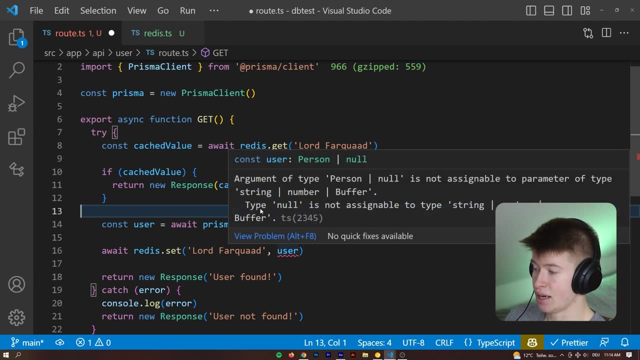 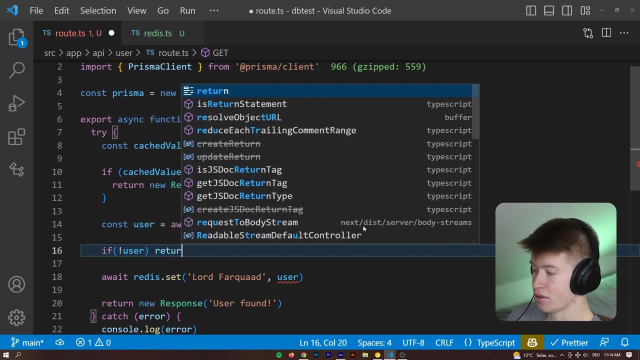 that's how we put values into a redis cache and then let's have lord farquad as the user result that we have gotten back and now the user might not exist. so we need to implement a guard clause here. if there is no user value, then we are going to return a new response of error. for example: 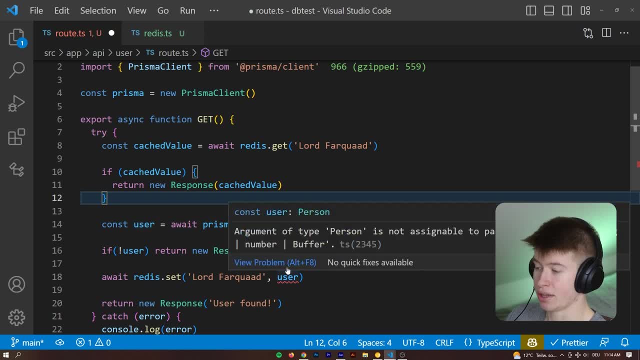 because this user does not exist. that way, we can ensure that this user right here that we are trying to put into a redis store is of type person. and the reason this is still giving an error is because we probably need to say jsonstringify and we need to say jsonstringify. 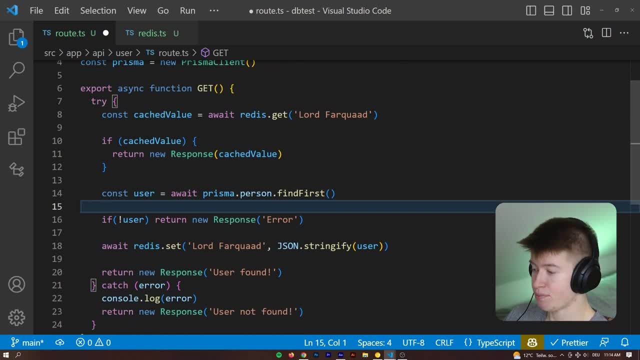 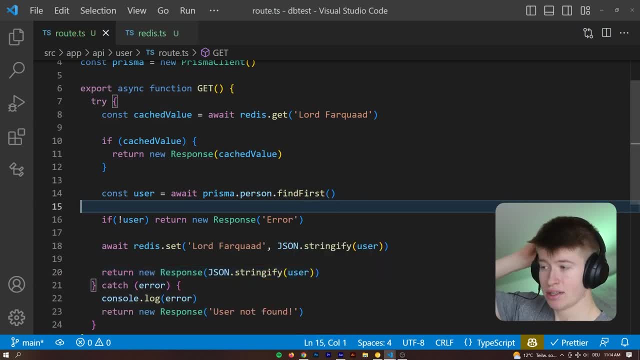 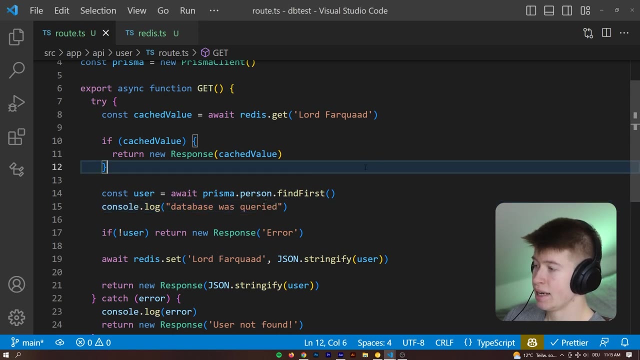 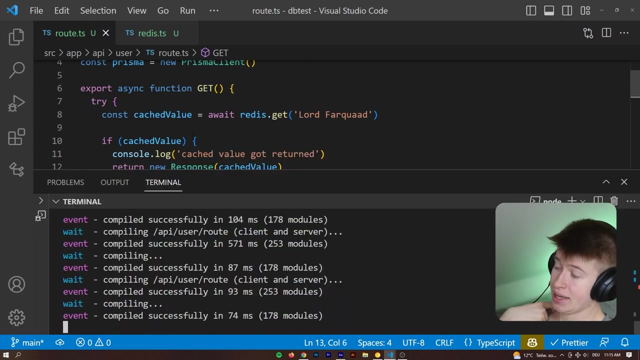 pass the user in here. so that means the first time we try this. the lord farquad is not gonna be in or redis cache, right, so the database will be queried. we can check that by just logging it out. database was queried and if the cache value was returned we can say console log of cached value got returned and that. 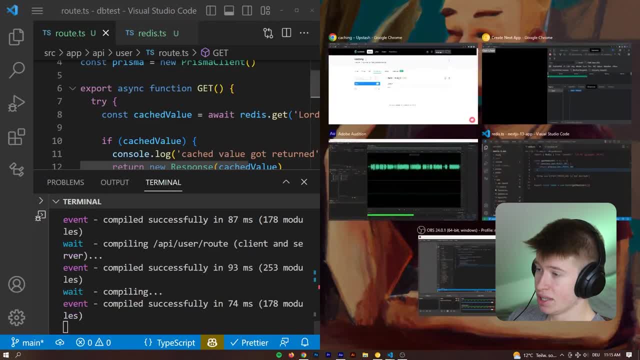 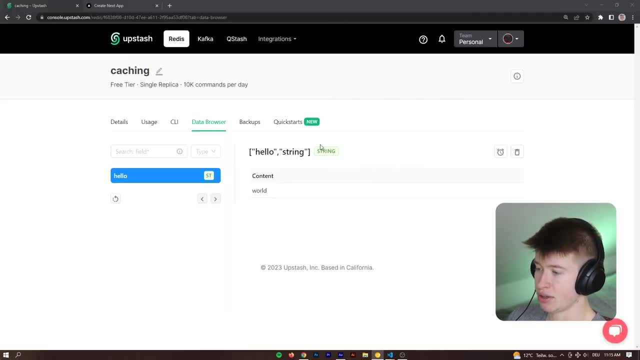 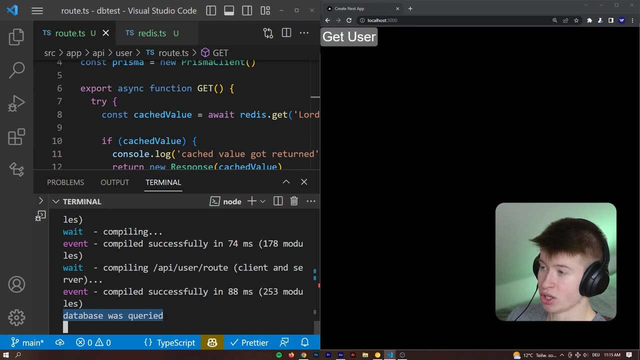 way we can see exactly what happened on the back end. so let's move this over into a side-by-side view again and let's click the get user. let's see what happens right here in the console. oops, let's go back into here. and we can see that the database was queried, obviously because the value 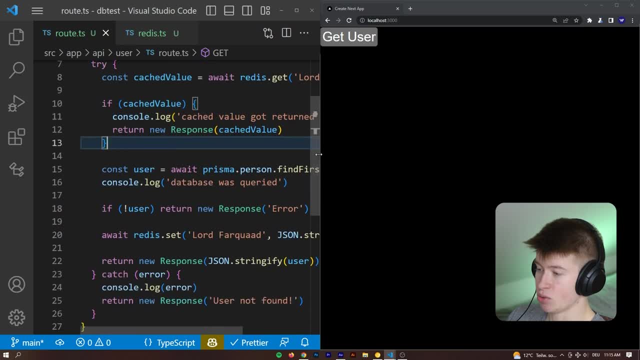 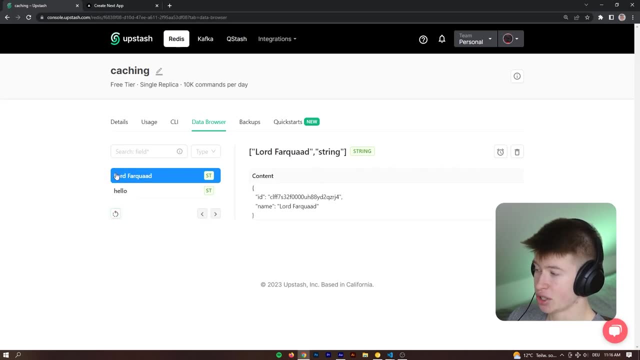 wasn't in our cache. however, we can see that the database was queried and we can see that the value was in our cache. however, if the database was queried, then we set it into our cache. so it should be in our cache, right? let's check the cache, let's refresh this, and we can see, lord farquad.